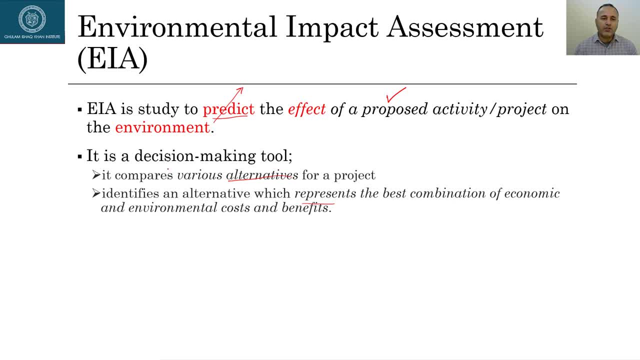 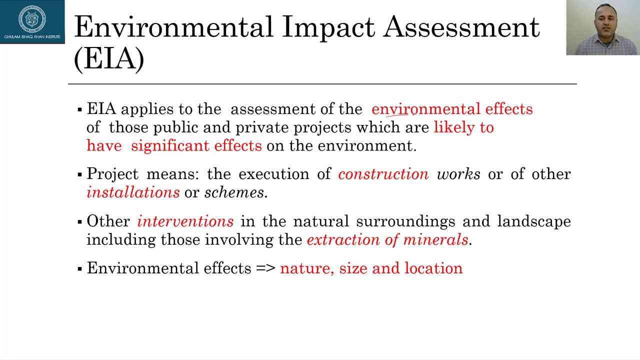 negative externalities. What environmental impact assessment does? it compares various alternatives and, based on your evaluation, you pick the right alternative. and from right alternative, what I mean is the alternative which is the best combination of economic and environmental cost and benefits. Now EIA applies to the assessment of environmental effects of those. 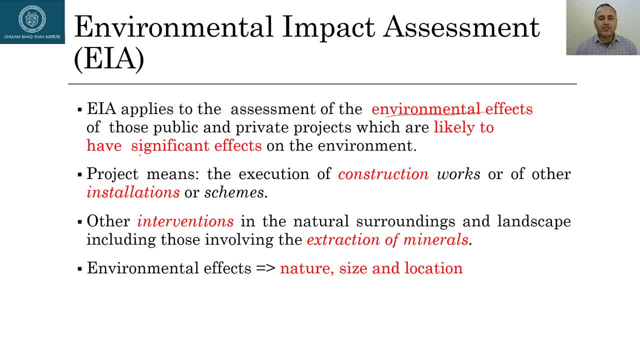 public and private sector projects which are likely to have a significant effects on the environment. So the purpose of this bullet point is that in countries like Pakistan, environmental impact assessment are not done for each and every project. They are done only for those projects which may have a 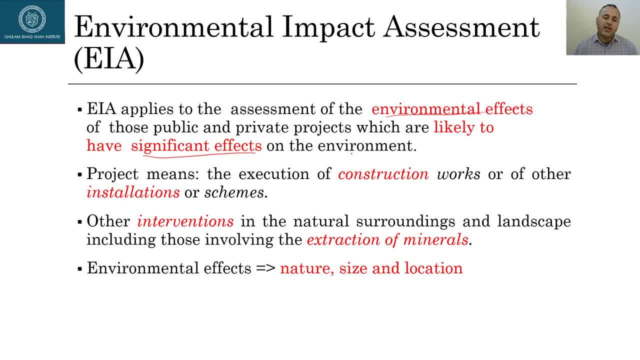 significant impact on the environment And, as you will see from the last part of this lecture, that there are some projects okay in certain sectors. of course they need actually all of them. they need environmental impact assessment. So not every project needs environmental impact assessment, but environmental impact assessment studies. 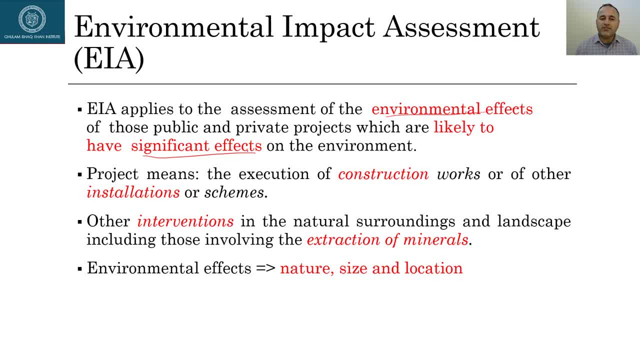 are normally done for those projects which have a significant effects on the environment. Now, project can be any construction project. so execution of construction works or any other installations, Okay. So projects normally entails construction work or installations, Okay, other interventions in the natural surroundings or landscape, including those willing the extraction. 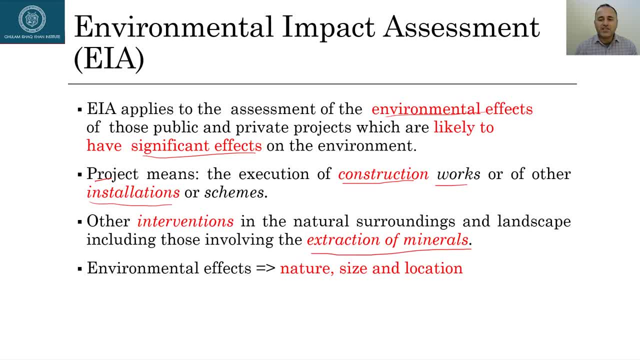 of minerals. Okay, so, beside construction works and installation, extraction of minerals, Okay, some areas, it is kind of an intervention. okay, so you are trying to actually what is called modify the ecosystem of a certain area, okay, by extracting the minerals. so impact evaluations, environmental impact assessments, are: 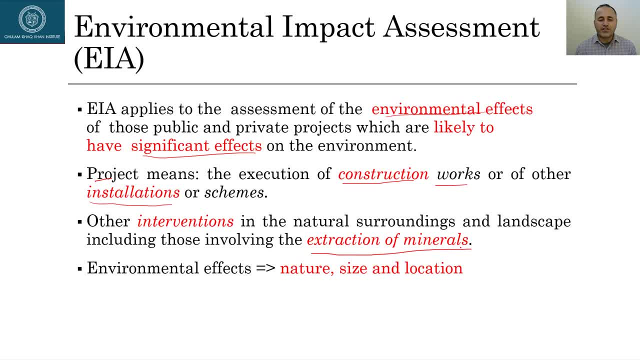 also done for those projects which involves extraction of minerals. okay, the environmental effects? okay, so what we need to know is actually the nature of the environmental effect. okay, so, for example, is the negative externality in terms of co2 emission or is it, let's say, the in the form of industrial waste, or 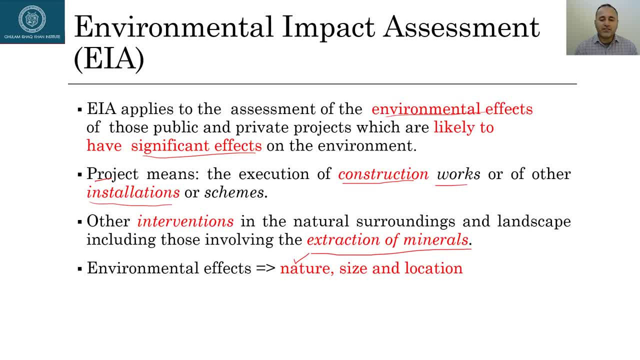 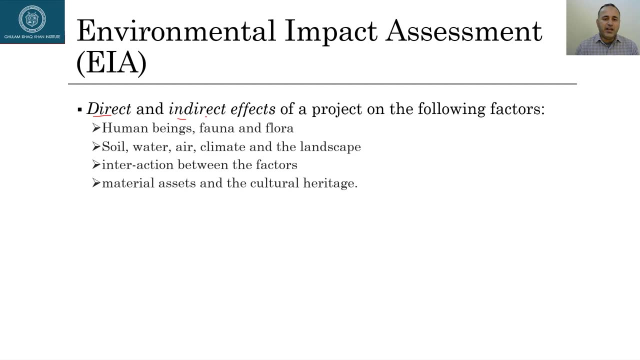 chemicals: okay. environmental effects also means like the size of the problem and the location. okay, so it's nature, size and location. direct and indirect effects of the project on the following factors: okay, so there may be some direct and indirect effects. okay, on human beings, fauna and flora, which is like the animal kingdom and the plant. 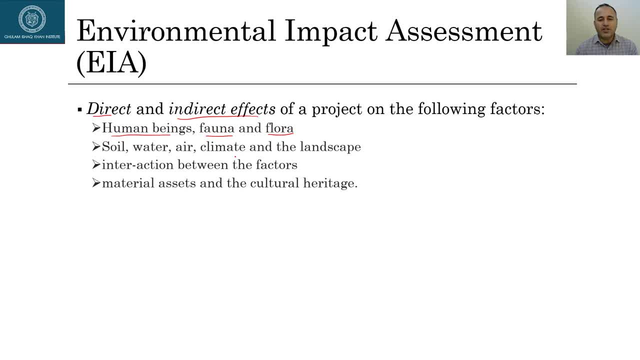 kingdom. soil, water, air, climate and the landscape- okay, and interaction of all these factors- okay. and it also involves material assets and the cultural heritage. so, for example, in countries, for example in Canada, there are some indigenous communities. so whenever a government tries to start a project in those 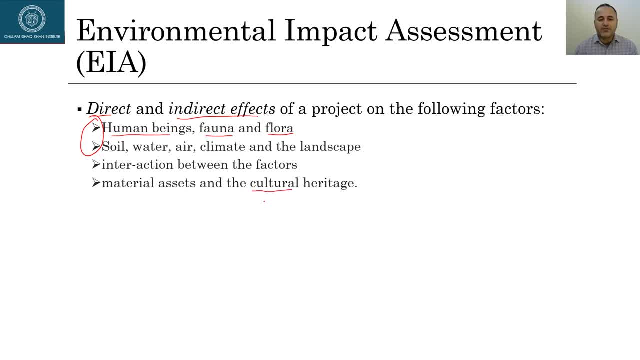 indigenous communities. they conduct a project that includes in their as the environmental impact assessment okay. so, for example, if a country try to visit the bathroom and a person gets На chercher problemas and on their immigration process, they don't simply show up in the morning that you want to do and that's what they do, and those have some. 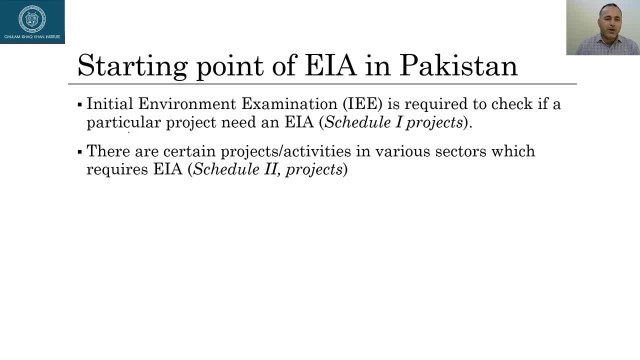 factors that may play a role in the environmental impacts. that's why the environmental impact assessment is important, right? so? thank you, LaMonte, thank you for sharing this so you can much need to these buildings, those the assessment. okay, So those projects are included in Schedule 1, okay, Everything included in Schedule. 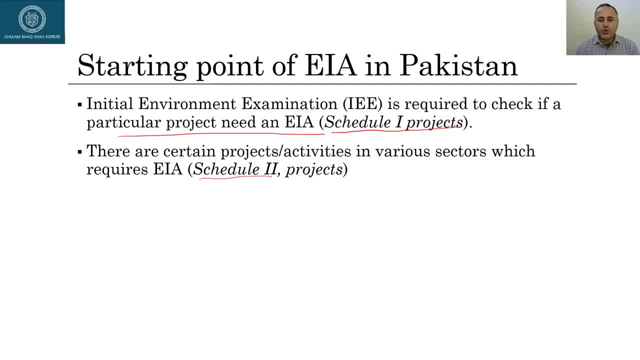 2, they need environmental impact assessment For Schedule 1,. what you do? you conduct an initial environmental examination. environment examination okay, And based on the finding of this initial environment examination, if it warrants further assessment of the impact, you conduct a complete. 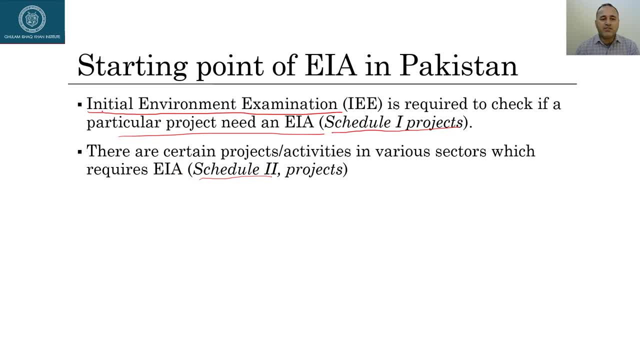 environmental impact assessment. okay, But let's say, if this initial environment examination suggests that the full-scale environmental impact assessment study is not required, then of course you do not carry out that study. okay, So in Schedule 1, projects, initial environmental examination is done. 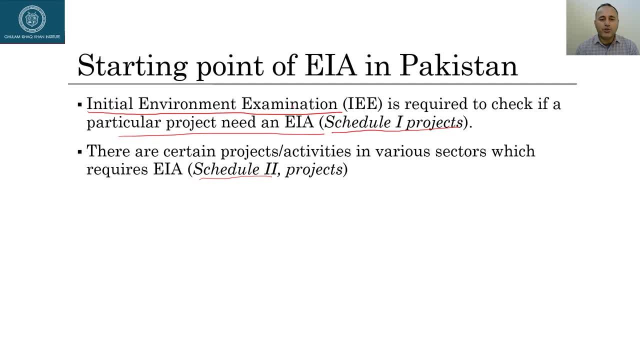 Okay, And based on the finding of that report, you either conduct the EIA or you just ignore it. okay, So it really depends on the recommendations of the initial environment examination report. Schedule 2 projects, though each and every project requires environmental impact assessment. 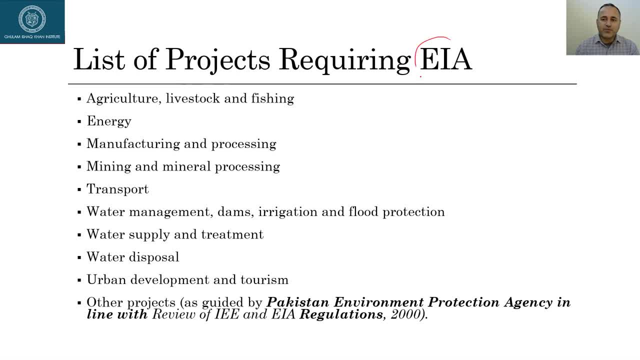 Now list of the projects which requires environmental impact assessment: agriculture, lifestyle and fishing, energy manufacturing and processing, mining and mineral processing, transport, water management dams, irrigation and flood protection, water supply and treatment: okay. water disposal- okay. urban development and tourism: okay. All these projects need. 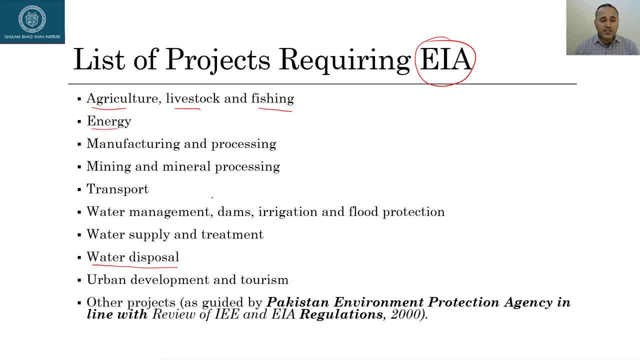 environmental impact assessment. In countries like Pakistan sometimes what really happens that some projects need environmental impact assessment. okay, So in countries like Pakistan sometimes what really happens is that some foreign and international donors are involved in these projects, So they are actually providing funding for these projects, For 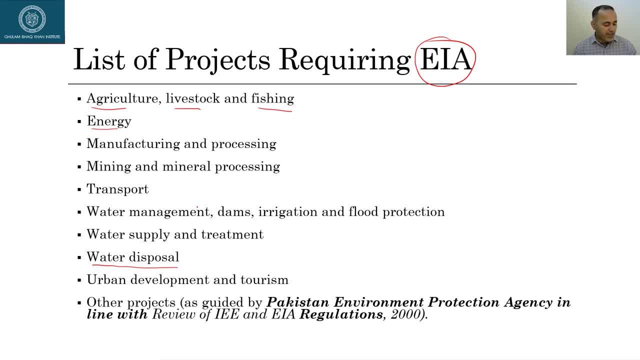 example, World Bank or Asian Development Bank. So one of the requirements of those donor donor- actually they, they, they give us loans of those lending institutions. One of the requirement is that we have to conduct environmental impact assessment. okay, 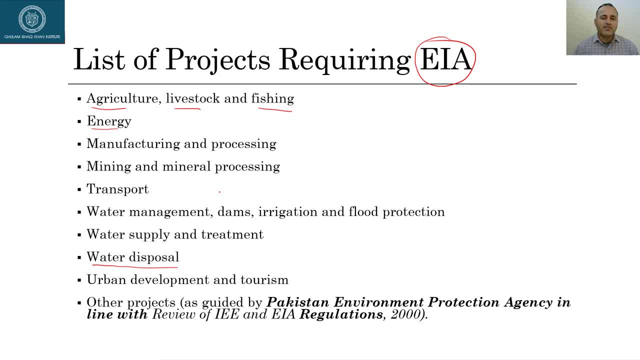 Sometimes it is also the, the- the requirement of EIAs- spray and pond over that we have to face environmental impact assessment. okay, Sometimes it is also the the the requirement of EIA as well, that the EIA�. 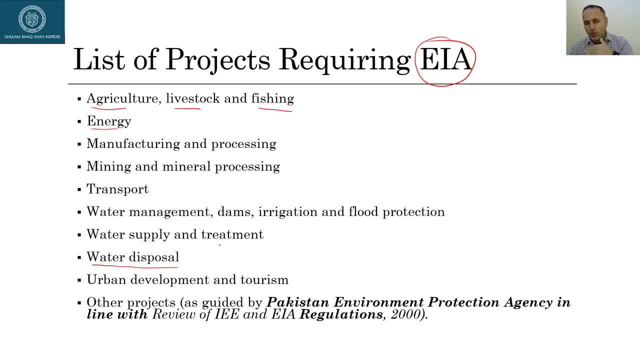 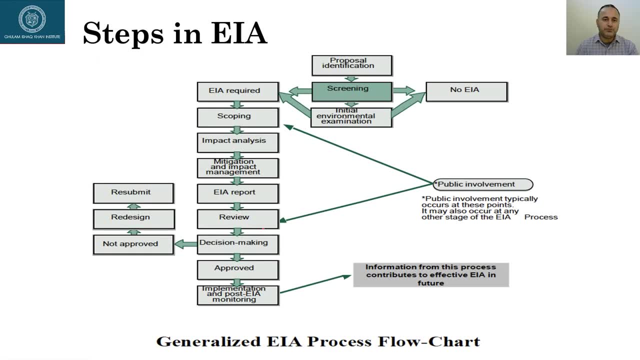 So EIA is alsoение the equivalent that we consider inGreen Tri experimentation, okay, Okay. So what is Kombata's final? also coming from the either donor or the lender. now, these are the key steps in environmental impact study assessment. okay, so everything starts with proposal. 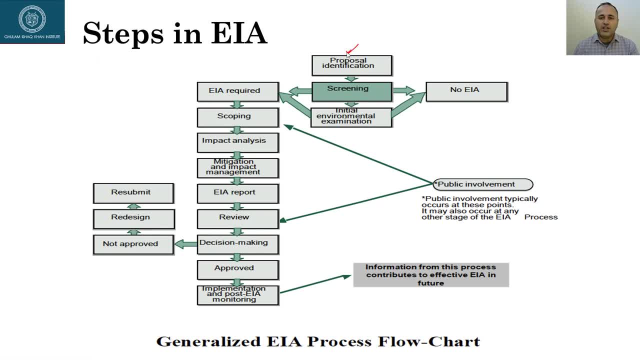 identification: okay. so let's say, if a government, whether municipal government, provincial and federal government, if they would like to start a project, okay, normally it start with the proposal stage. okay, that proposal is screened, in other words, it is evaluated. okay, and if the EIA is required, okay, so you. 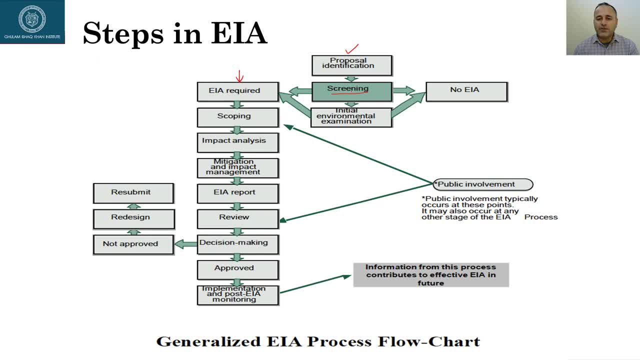 start here. okay, but some of the project, as I told you in on one of my slides. okay, if the project is in schedule one, okay, it does not necessarily require EIA. okay, So you conduct initial environmental examination If based on initial environmental examination. if no EIA is required, that's fine, you just 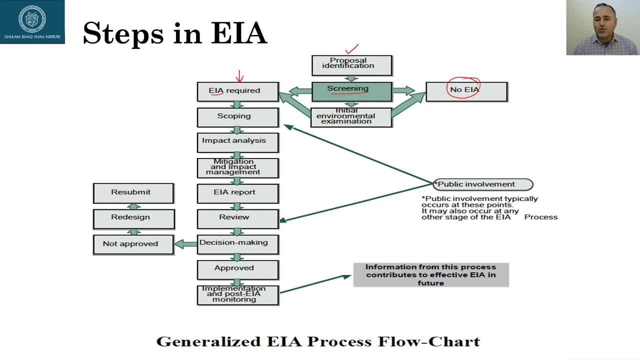 stop here. But let's say, if the IEE, which is the initial environmental examination, if it suggests that it needs EIA, so you start this process here. So if we, whenever we establish that the environmental impact assessment is required, the next stage is scoping, and I'll talk about what scoping actually entails. 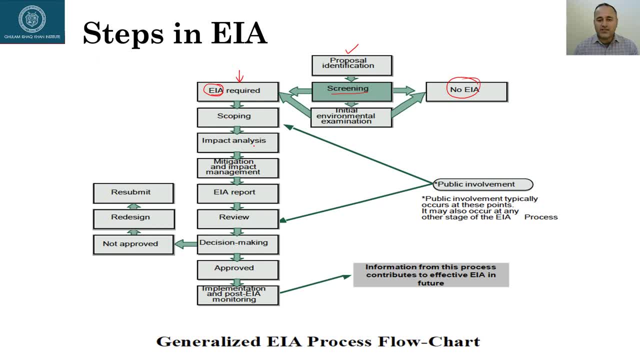 Then in the next step we do impact analysis and in the impact analysis we also include mitigation and impact management. All these components actually form the EIA report. The next stage would be review, so a regulator or the public actually reviews the report. 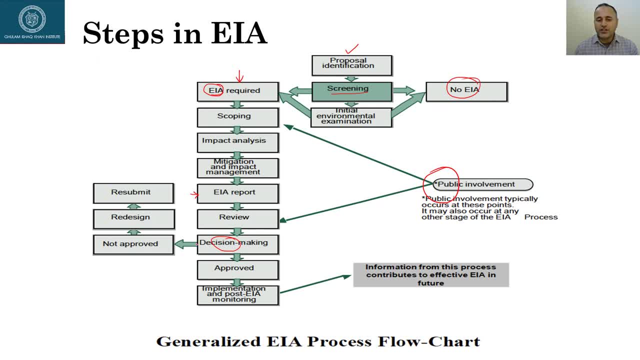 and then the EIA reports. They make a decision. okay, So the decision can be either approved, which is here, or not approved, okay. If it is not approved, okay, you cycle back, You redesign the project and resubmit it for evaluation. okay. 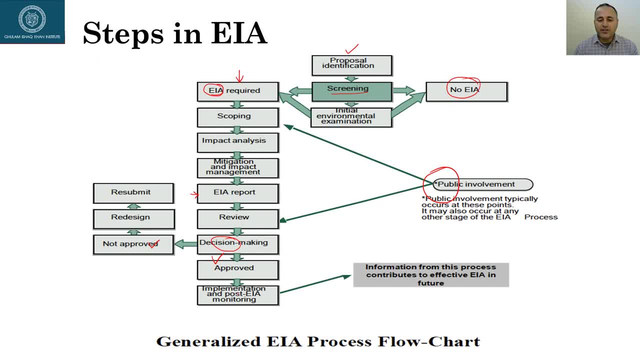 But let's say, if the decision is that the project is approved, then of course you go to implementation stage and post EIA monitoring. okay, Now the involvement of public. As I was talking in my presentation In my last lecture, it is extremely important okay. 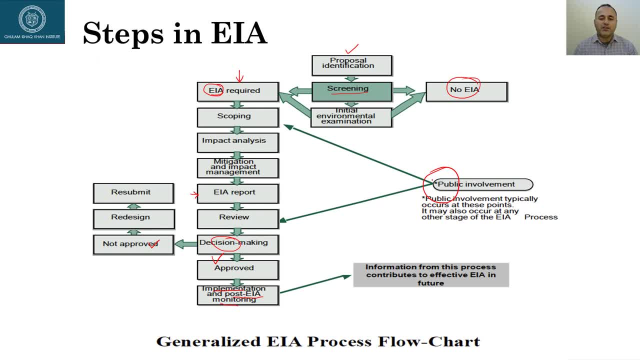 It really helps public- not okay, let me choose my words properly- So it creates actually ownership among the public for the project. okay, And the people think that okay, whatever the project is being carried out, the government or, let's say, the private company, they are really valuing their feedback. 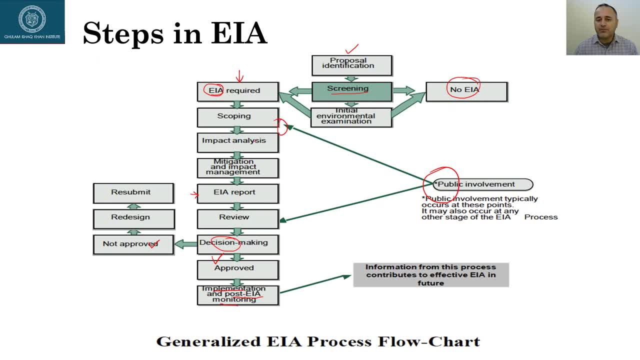 So the public involvement Or feedback can be either involved in the scoping stage or in the review stage, But there is no rule of thumb. You can actually involve public's opinion in the scoping stage as well as in the review or in one of these. okay, 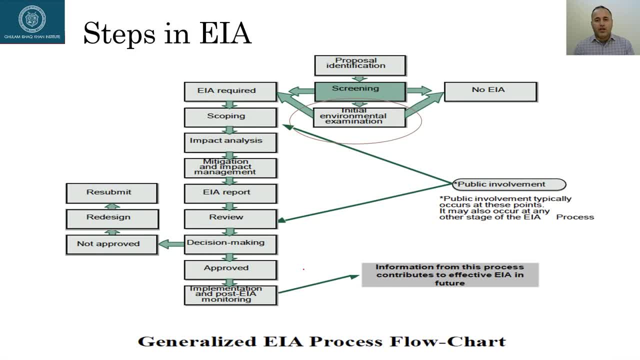 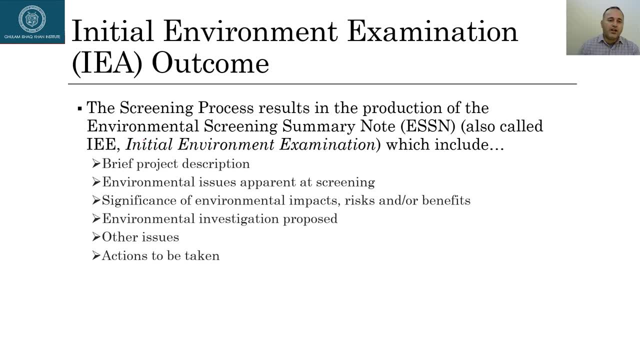 So there is no rule of thumb, okay, So let's talk about scoping, initial, actually environmental examination. So the screening, The screening process, results in the production of environmental screening summary note. okay, So forget about these jargons, okay. 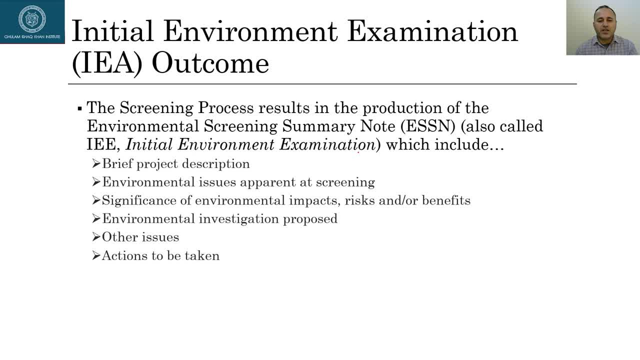 The most important thing is that the initial environmental examination. it includes brief project description, So it describes the project okay. Environmental issues apparent at the screening: okay, So they highlight the environmental issues, okay, involved in this project. Significance of environmental impacts, risk and or benefits: okay. 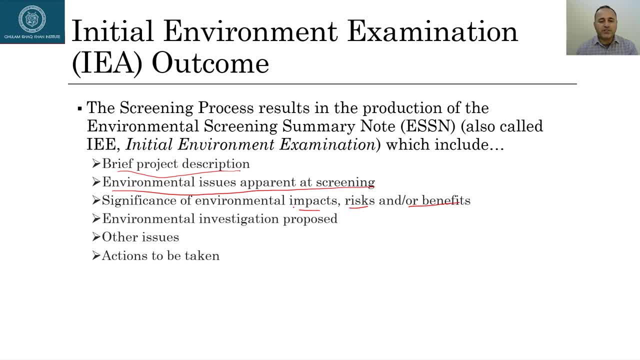 So the significance of environmental impact, risk and benefits are also highlighted in this report. okay, And the environmental investigation is proposed. If it is proposed, it means that we have to go to environmental impact assessment. okay, It also let's say: any other issues can also be highlighted. 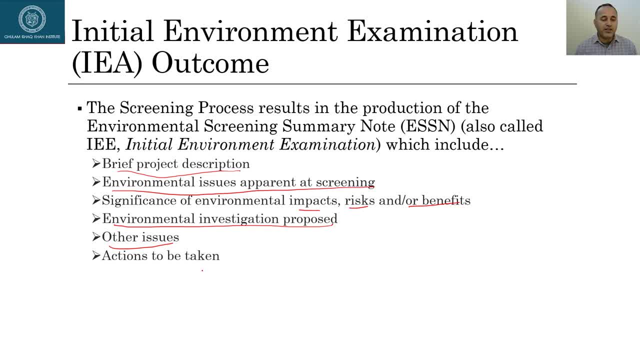 Okay, So that's it, Thank you, That's it. And then, of course, it highlights the actions which needs to be taken. One of the actions may be that it actually recommends either the regulator, the government or the lender to carry out a full-scale environmental impact assessment study. 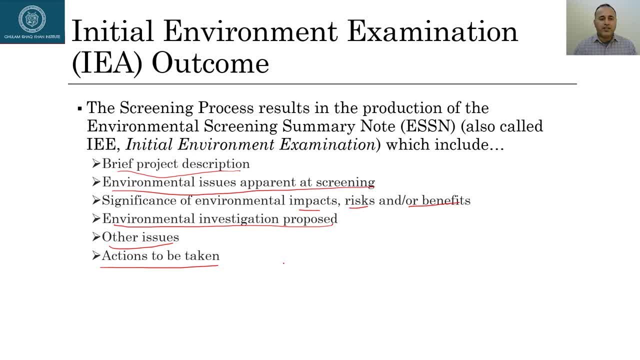 So, as I told you in one of my slides, that the initial environmental environment examination is done, Okay, This is not a schedule one project in Pakistan. okay, And if it recommends, okay, then we do environmental impact assessment. okay, The full-scale one. 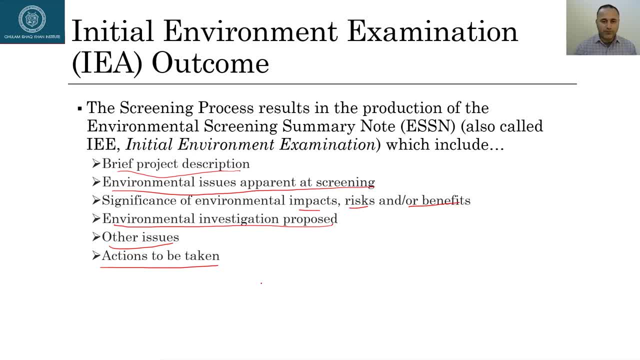 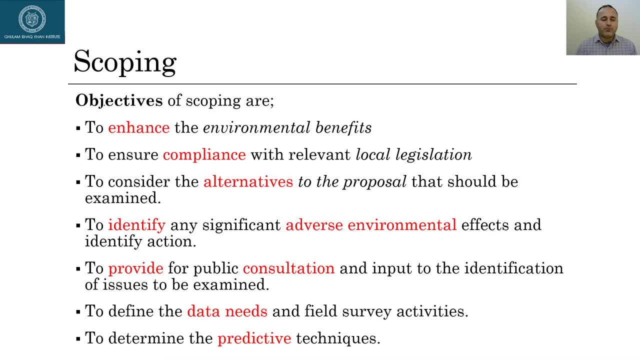 Now scoping. Scoping, and I'll read through it, because these are very, very easy to understand. okay, So the objectives of the scoping are to enhance the environmental benefits. Okay, So that's one of the main purpose. 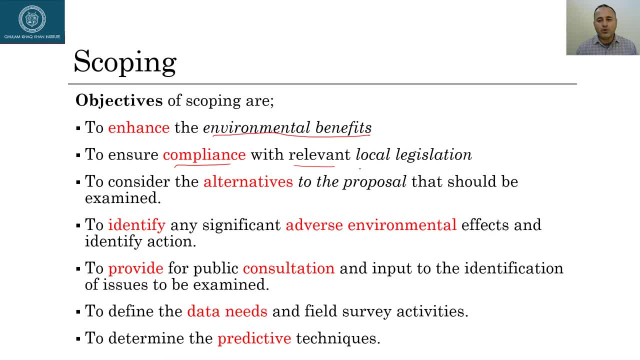 To ensure constitutional impact: focused and enhanced: Okay. compliance with relevant local legislation: okay. to consider the alternatives to the proposed: that should be examined: okay, so consider the alternatives to the proposal that should be examined, like, for example, if if the proposal in Pakistan is to, for example, build a railway track, okay, so we can. 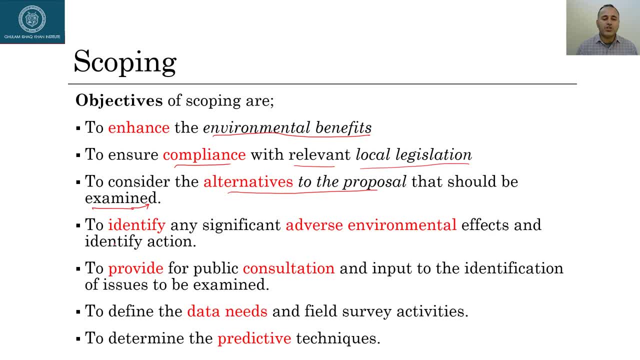 connect different cities. okay, so we can choose different routes. rate: okay, so the the scoping of the environmental impact assessment study. it also touch upon the alternatives. the proposal then okay. okay, we are, we are evaluating this proposal in terms of impact on on the environment, but there are some other alternatives. 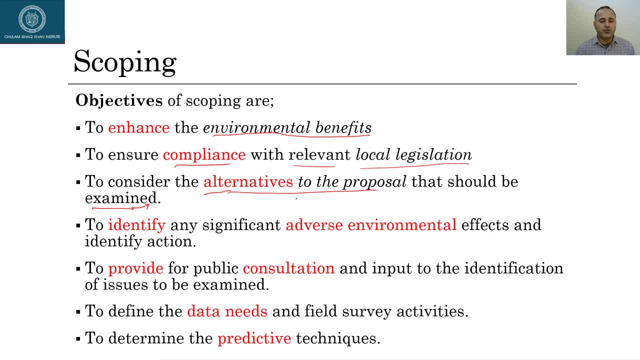 okay, so scoping may also consider alternatives to the proposal To identify any significant adverse environmental effects and identify action. So this is the mitigation part. So scoping identifies the adverse environmental effects, but it also identifies the corrective actions To provide. 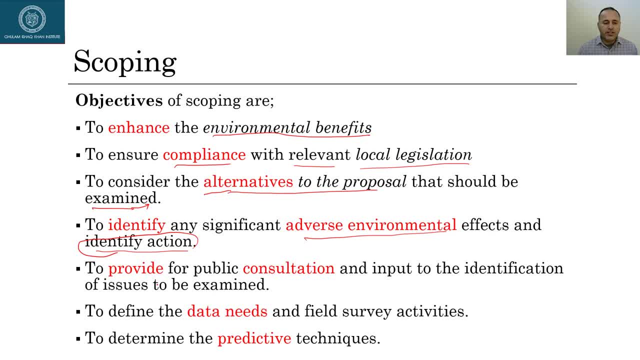 for public consultation and input to the identification of issues to be examined. So scoping actually provides an opportunity for the public to provide their input to define the data needs and field survey activities. Scoping actually defines the data needs. For example, what would be the impact of the proposed project In order to quantify. 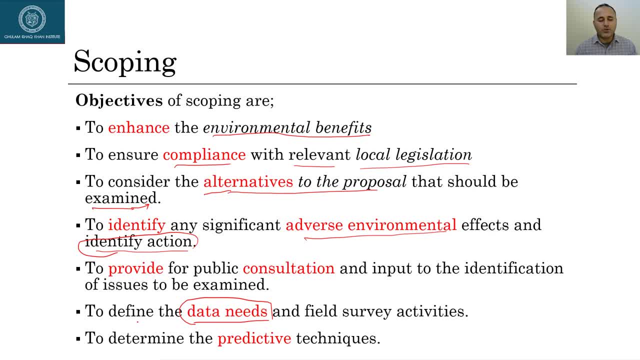 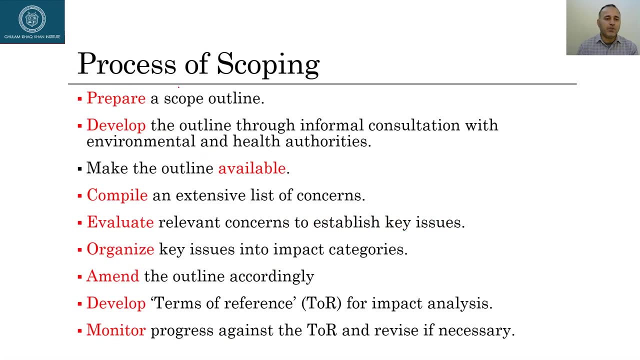 that impact. you need data- okay, so scoping actually defines the data to determine the predictive techniques and it also tells you about the techniques that the study is using for predictive analytics. process of scoping: okay, so prepare a scope outline- okay, develop the outline to informal consultation with environmental and 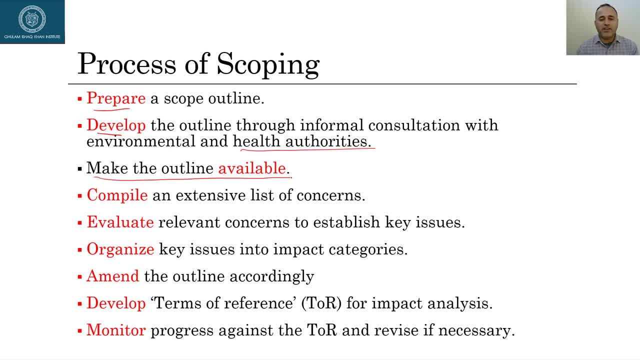 health authorities. okay, you make the outline available. okay, you make the outline available to the public, because it is extremely important that you get their feedback, not only from the public, but also from other agencies. okay, or companies compile an extensive list of concerns? okay, so this is like a 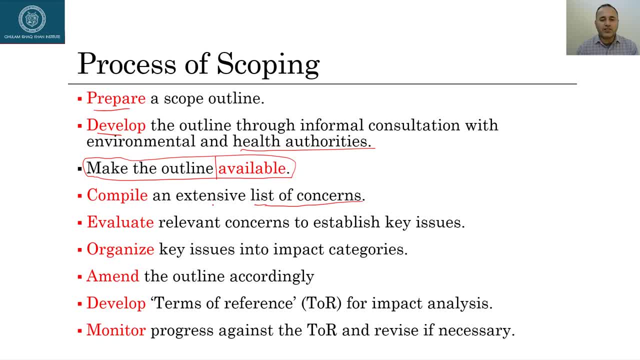 brainstorming stage where you compile extra extensive list of concerns, you evaluate relevant concerns to establish key issues. okay, so this is like more of a brainstorming step. okay, the evaluation part is more of an analytical step where we analyze all the concerns and then we identify the key. 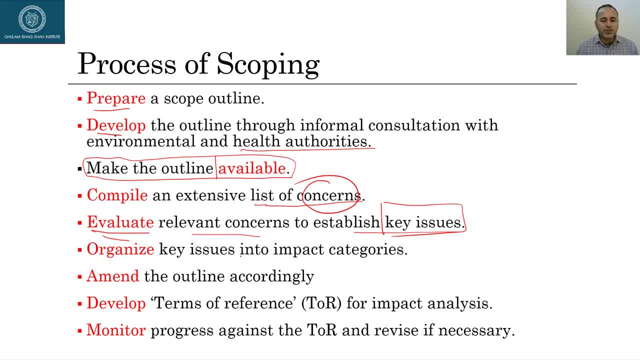 issues. organize key issues into impact categories- okay. amend the outline accordingly- okay, and develop terms of reference: okay, for the impact analysis and then you monitor the progress. okay, so terms of reference is extremely important. okay, so, based on the feedback that you receive from the public and other agencies: okay, we identify key issues. okay, we organize them and we then 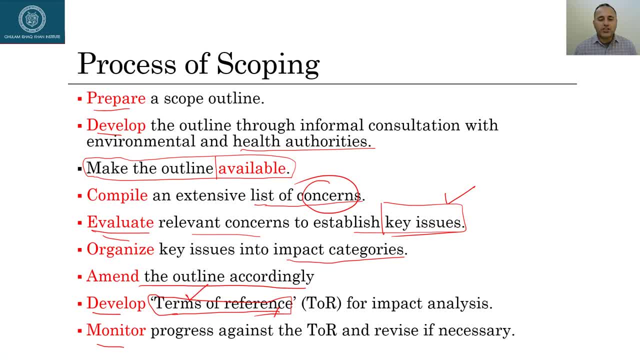 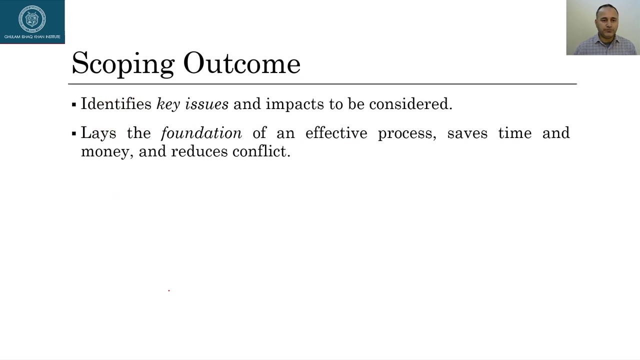 develop terms of reference. okay, so the terms of reference actually defines the scope of the project. okay, of course you have to limit the scope of your project, so terms of reference is really about actually defining the scope of that project. now, the scope outcomes. what does the scope scoping does so? scoping identifies key. 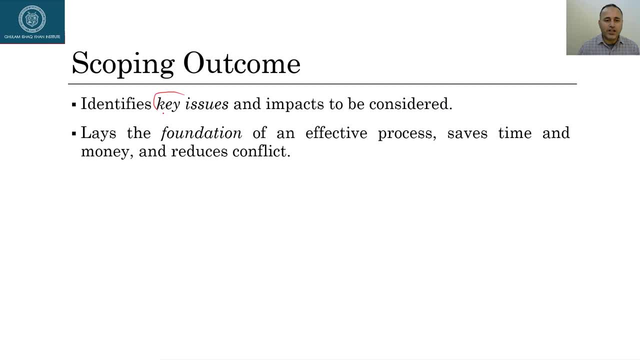 issues and impacts to be considered. okay, so it actually identifies key issues and impacts. okay. it lays down the foundation of an effective process, saves time and money and reduces conflict. okay, because once you identify issues, once you identify the potential impacts of those issues- okay. and once you suggest: 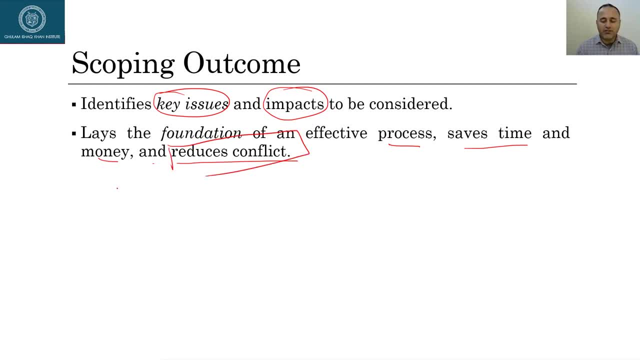 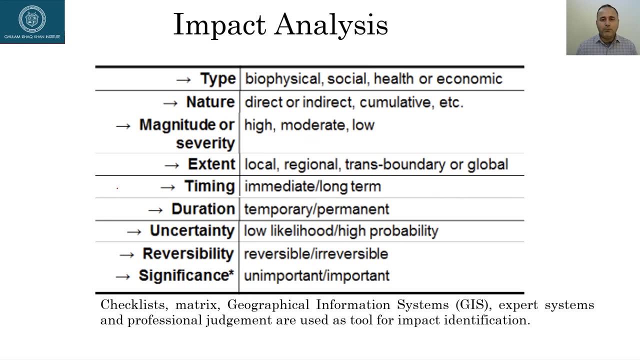 corrective actions. it reduces the chances of any conflict. now impact analysis. now impact analysis. ok, whether the impact is biophysical, social, or is the impact, let's say, in terms of health or economic loss, or economic gain? economic loss or economic gain, again ok. and what is the nature of impact? is a direct or indirect or cumulative? 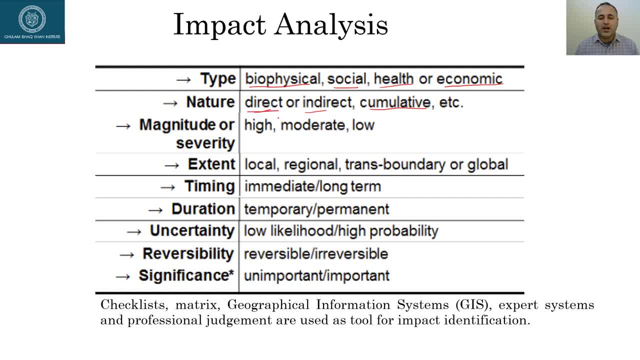 okay, so sometimes 932 0932 0031 cannot see the direct impact of a certain project. okay, but it has some indirect implications okay, especially in the biophysical space. okay, because these projects has some long-term impacts. okay, and it can certainly, for example, endanger some species. Let's say, for example: 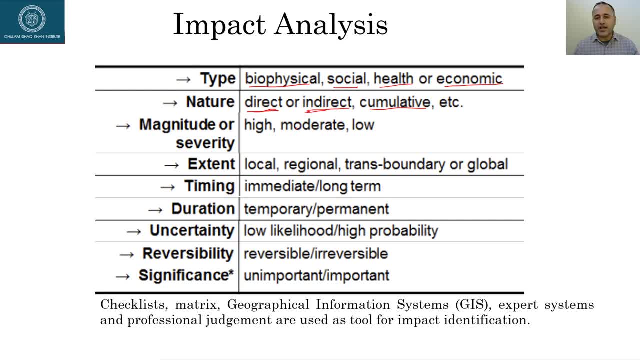 if we are talking about large projects like dams, okay, or even highways, okay. so it may have a direct or indirect implications on the different habitat or biophysical space, okay, and what is the magnitude of that impact? So, based on their experience, actually, they categorize them as high. 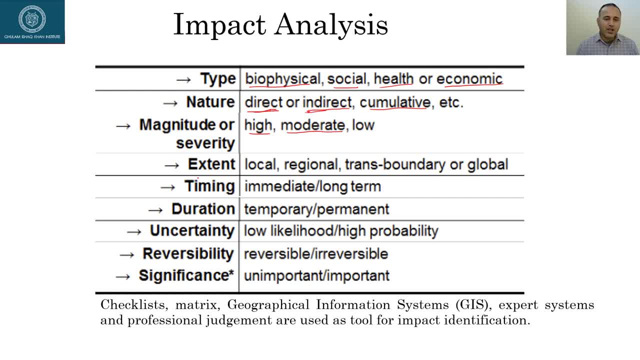 low or moderate, okay, Extent okay. so is the impact? okay, are the implications local, regional or transboundary? So I was talking to you about a gas pipeline between US and Canada. Now that particular project has transboundary okay, implications okay. so the implications are not limited to. 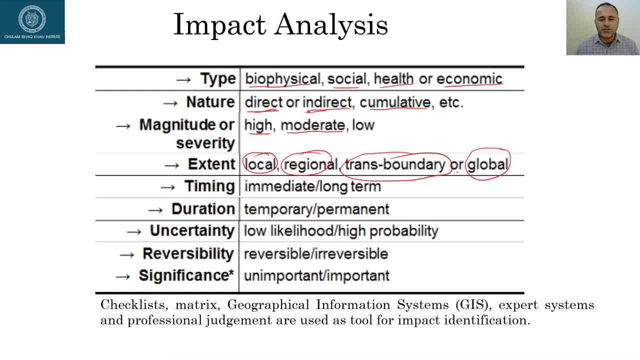 one country, okay, and it may have some global implications as well. Timing so is the impact itself. is the negative or the positive effects realizable immediately, or will these impacts be in the long term? okay, and are these like? 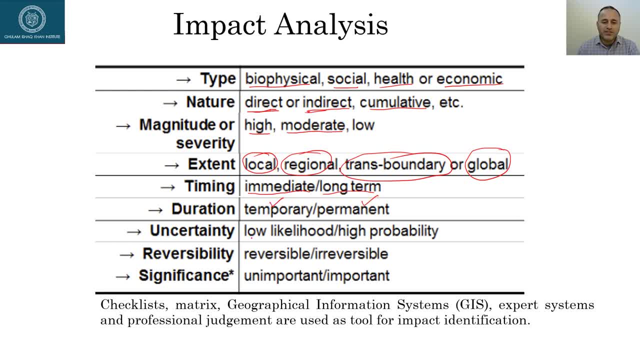 let's say temporary or permanent: okay, and uncertainty, okay. for example, a certain, let's say, negative impact, For example: how likely is that? okay, what is the likelihood of that? So, for example, if I think we had a, 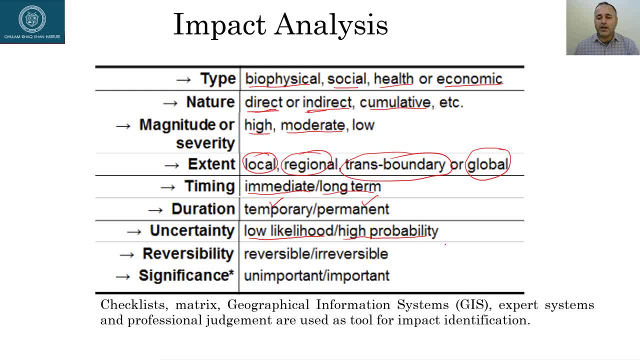 big issue, in my opinion, that was in Japan because as a result of earthquake, one of their neutral plants actually had developed some serious problems okay. So although those nuclear plants, I'm sure they must have done, they must have worked okay, for example in the UK or also in the United States. 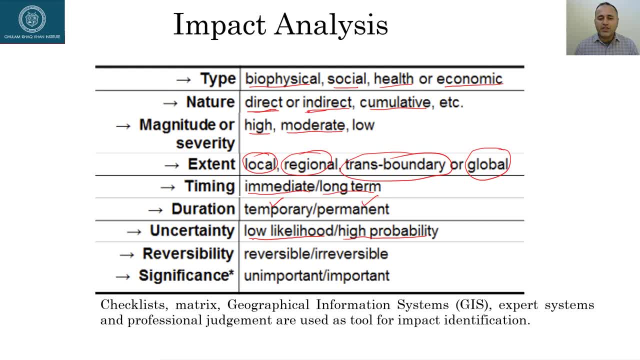 they must have worked for highly advanced nuclear resources. okay. So these are. they are very, very high scientific features of the environment, environmental impact study and the chances of whatever happened as a result of that earthquake. it it might have been a low likelihood event, okay, but things 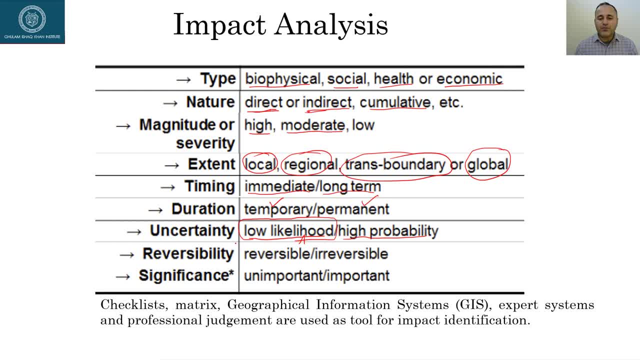 happen, okay. so once you identify something in the environmental impact assessment, okay, you also assign the probability to it, whether it's a low likelihood event or is it a high probability event, okay, reversibility are the negative effects- let's say reversal- or they are irreversible in nature- okay, because these will have different implications. 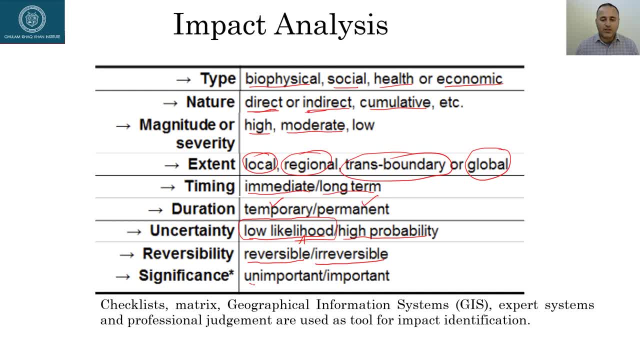 okay, significance is: are they significant? okay, so, from significant means, are these events, let's say, important or less important? okay, so, from significant means, are these events, let's say, important or less important? okay, now checklist matrix. okay, geographical information system, expert systems and professional judgment are used as a tool for impact identification. okay, so we use all these three tools. 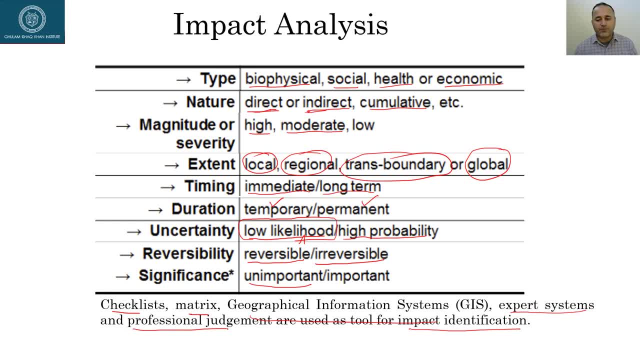 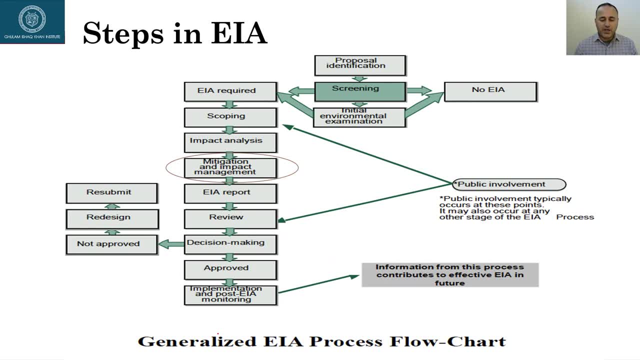 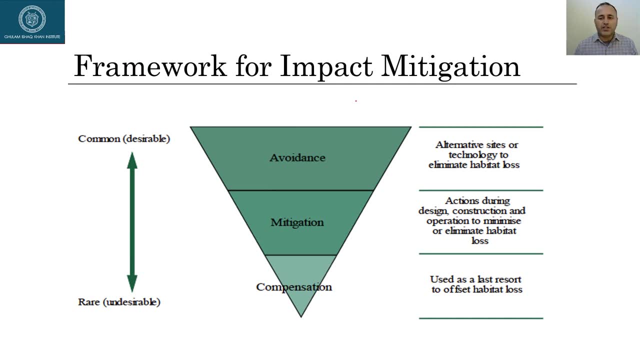 including professional judgment: okay, for impact identification. now mitigation and impact management. now, framework for impact mitigation avoidance: okay. so alternative sites or technology to eliminate habitat loss. so, as I was talking to, let's say, if a government, whether provincial or federal government, if they would like to, let's say, build a dam, okay, and the environmental impact? 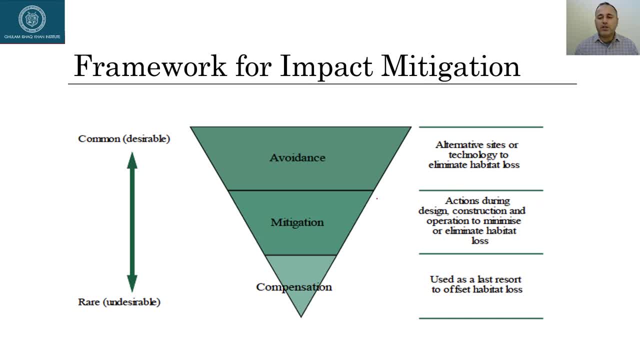 assessment study suggests that the impact will be huge in terms of, let's say, habitat loss. okay, so your next question is: can we avoid this particular project? okay, you just, let's say, change the site of your project or you do some modifications, so you try to find out whether 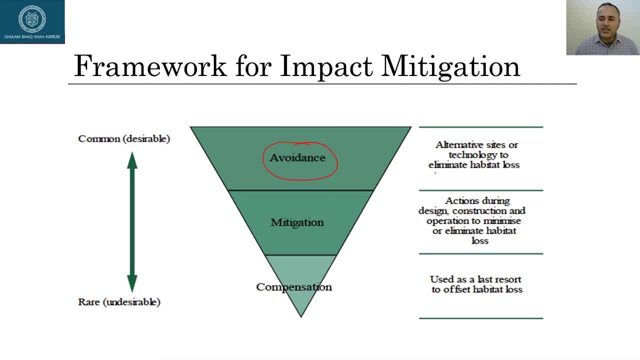 alternative sites or technology is available to eliminate the habitat loss? okay is the loss of avoidable in that way? in other words, okay, now actions during design, construction, integration to minimize or eliminate habitat loss? okay, so yes, you identify habitat loss, okay, you acknowledge it, but now you try to provide some mitigation strategies. okay, so avoidance is. 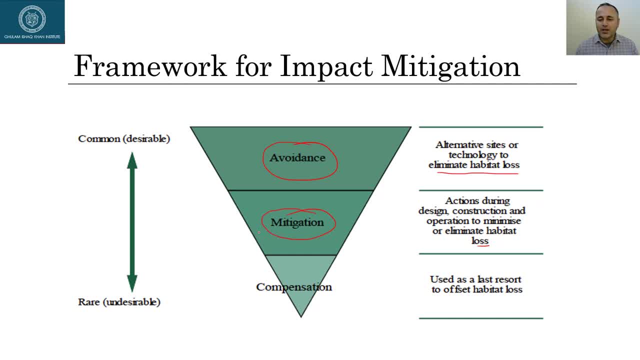 not an option you are trying to avoid, because if you avoid that little bit and reward the type of loss, then sometimes that can get lost. that could be a very large amount. so let's say a project which to mitigate it now okay, in other words, you are trying to minimize its impact. 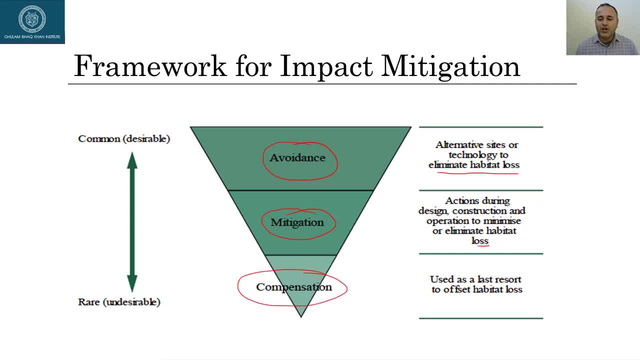 okay, compensation. okay, what really does? it's used as a last resort to offset the habitat loss. okay, so you provide compensation. so, for example, in social sphere, if a dam is resulting in, let's say, loss to somebody's property, for example it's a physical property, house or anything- okay, what you do? you provide. 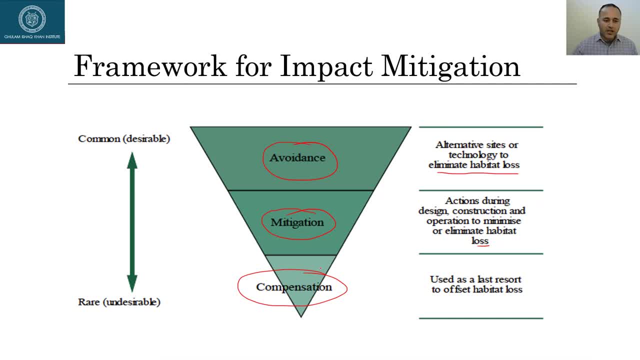 compensation to them. okay. now, moving actually from down to up: okay, this is a more desirable area. okay. anything which can be avoided, of course, it is more desirable, okay, but things which cannot be avoided, then you provide compensation for them. okay, and it's a لا. let's see another interestingVESHA. 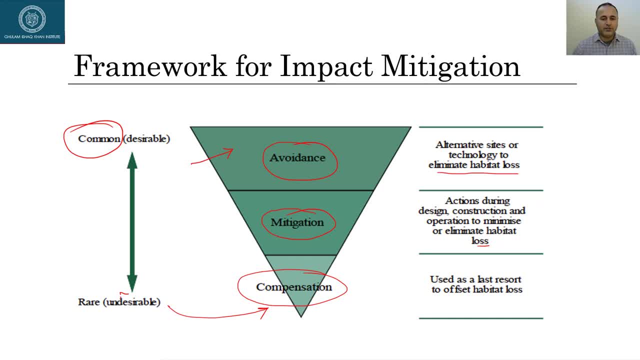 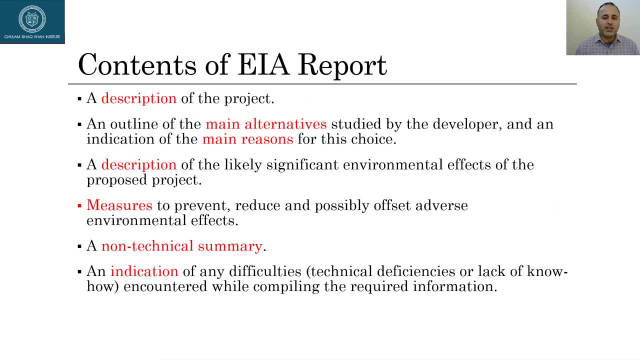 think we will simply say, the panting being very aggressive: yeah 🎜. so don't get angry at me for innocent someone. 🎜 really okay to say I'm so sorry, okay, okay. less desirable situation: okay, okay. the EIA report, now the EIA, the environmental. 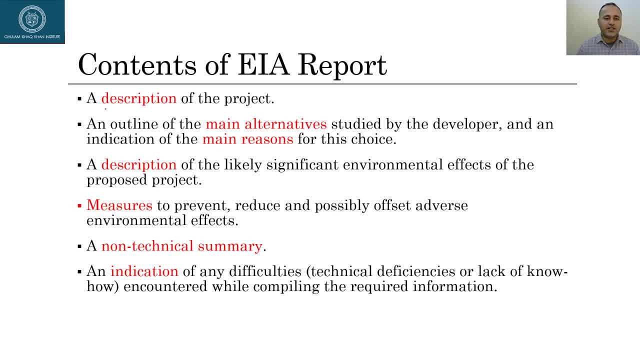 impact assessment report. normally it entails the description of the project, so the project is described. an outline of the main alternatives. okay, so what are alternatives available to this project? okay, so an outline of the main alternatives studied by the developer and an indication of the main reasons for this choice. okay, so it also highlights the areas where the main 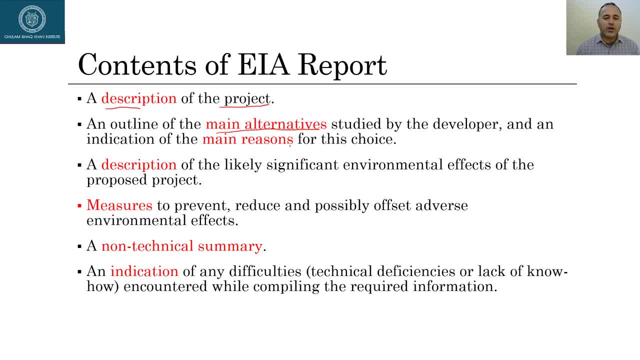 alternatives are described, okay, and then it also highlight those areas, the main reasons, actually that why this particular choice has been chosen, this particular alternative has been chosen- okay. a description of the likely significant environmental effects of the proposed project: okay, so you identify and recognize, okay, the significant environmental effects. okay, in fact, this is the main point of the EIA. 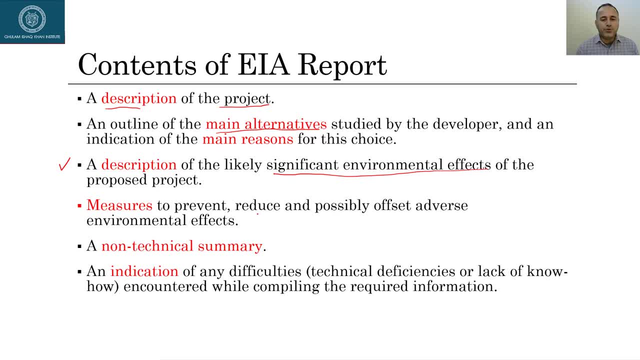 report. okay, you measure to prevent, reduce and possibly offset the adverse environmental effect. okay, so either you try to prevent- okay. in that case it will be like avoidance. the reduction would be mitigation and possibly offset the adverse environmental effects. this would be the main point of the EIA report. okay, 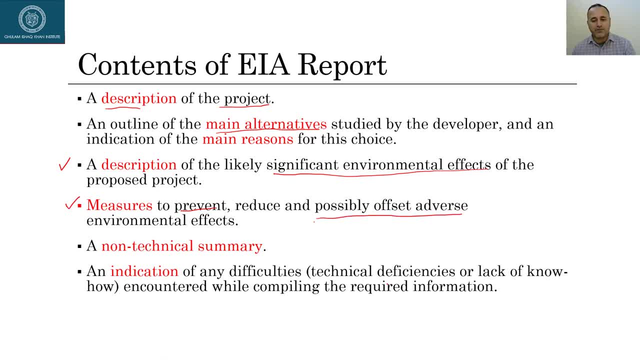 this would be the compensation part of it. okay, a non-technical summary. then, of course you since since one of the main reasons you are writing the environmental impact assessment report is actually to share it with regulators and public, so you also write a non-technical summary, okay, which is like: 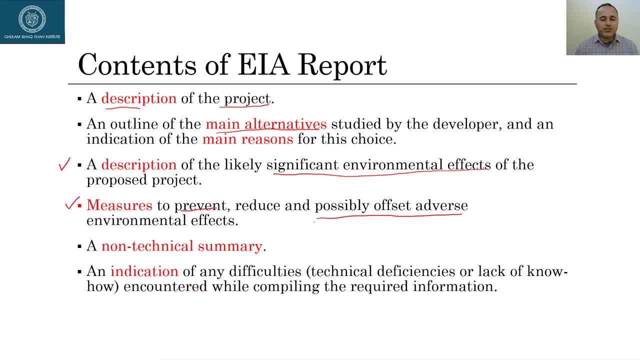 for consumption of junk public- an indication of any difficulties, technical deficiencies or lack of know-how encountered while consumption of junk public- an indication of any difficulties, technical deficiencies or lack of know-how encountered while compiling the required information. okay, so let's say if, as a consultant, if you.